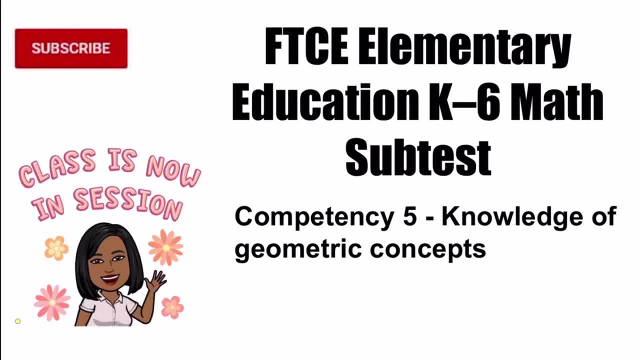 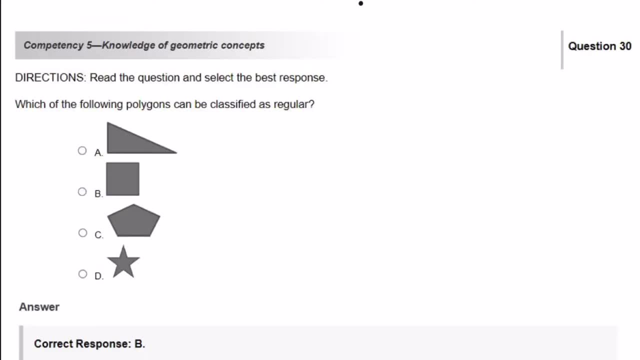 Welcome to Mrs Taylor's math class. Today's topic is FTCE- Elementary Education- K-6 Math Subtests, Competency 5: Knowledge of Geometric Concepts. Now let's begin class. Which of the following polygons can be classified as regular? So in order to solve this question here, you will first have 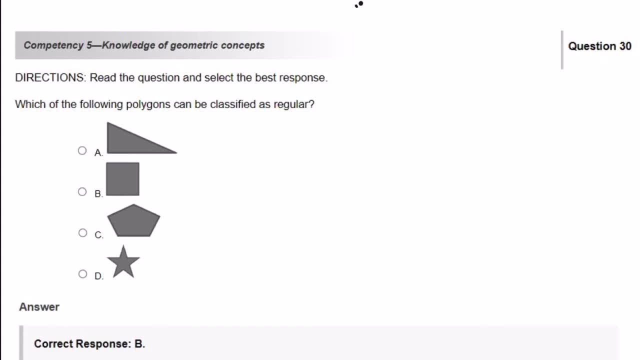 to know what regular means. So, when it comes to polygons, the word regular means a polygon in which all the sides of the polygon are the same length. So all sides are the same length, okay. And so, looking at the four pictures that we have here, we have a triangle, a square, a pentagon and a star. so, by definition, 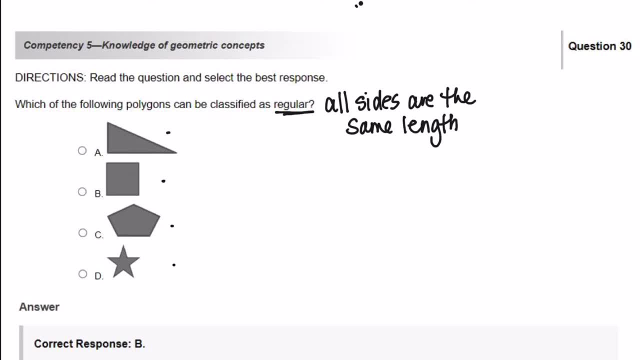 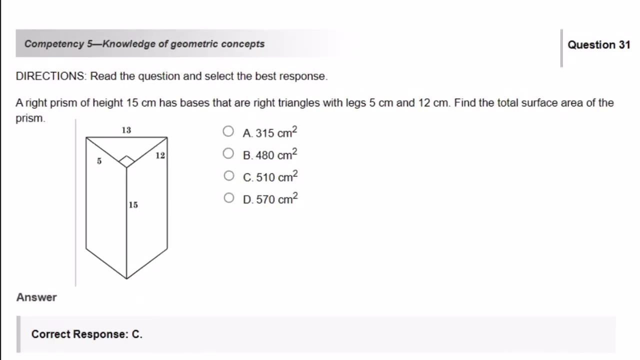 the polygon listed, all the polygons listed here um the square, is the only one that has um all sides the same length, just by definition. so we're going to go ahead and just select that. a right prism, of height 15 centimeters, has bases that are right triangles with legs 5 centimeters. 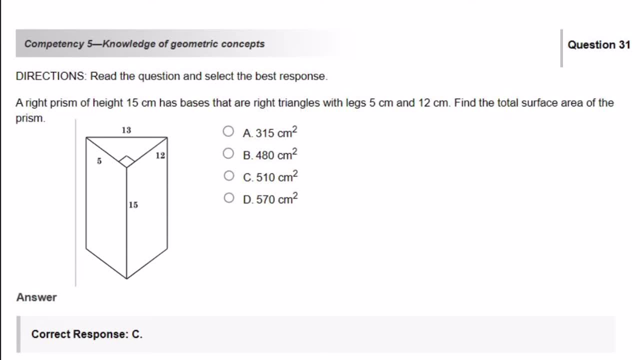 and 12 centimeters find the total surface area of the prism. okay, so this picture can be a bit confusing. so let's identify all of the different sides that we have to find the area for. so i'm going to draw um some additional information here to help you out. 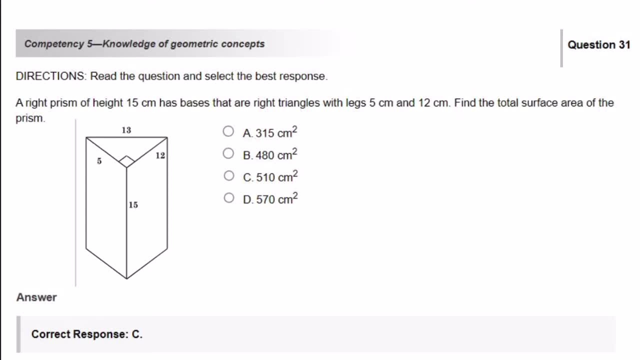 so we have what they call a prism, and a prism is um a three-dimensional shape that it has. bases are the same. now, i know this may be a little bit difficult to understand and to see, but i'm gonna try to help you out. so the base of this prism is a. 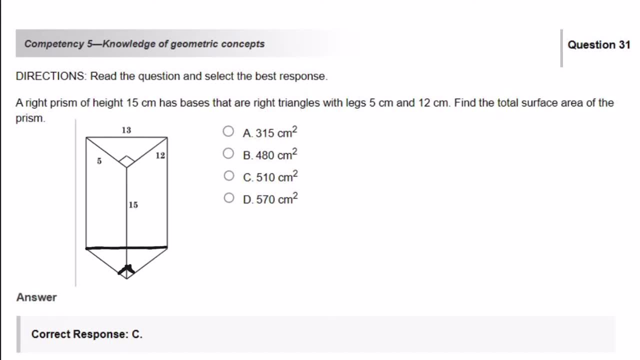 triangle. the base of this prism is a triangle because if you look at the top of the triangle which is here, well, the top of the prism which is, um, up here, and then the bottom of the prism which is down here, the shape is a triangle. okay, if i had to draw it without 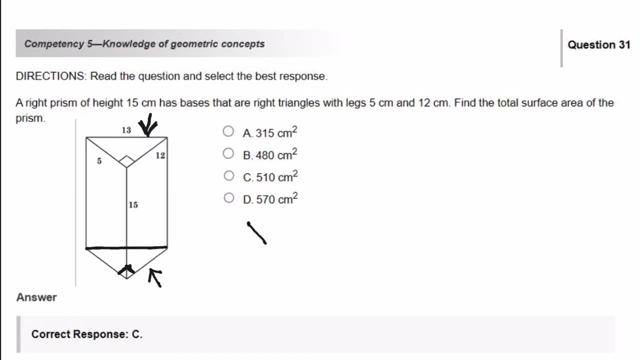 um, just to draw it, without everything, it would look like this, and hopefully this makes sense. so i'm drawing this and this is really what you have. so we have the two triangles and they have the same dimensions, meaning that they both have two legs and their lengths are five centimeters. 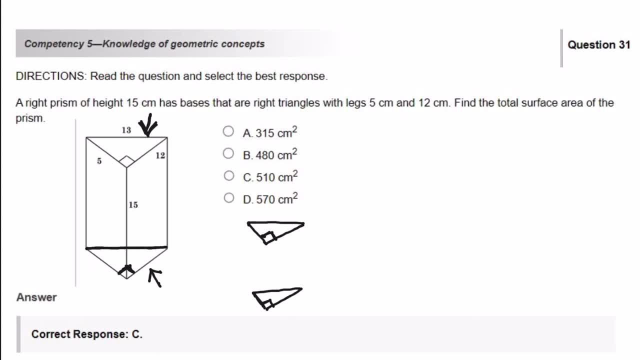 and 12 centimeters. so, in order to find the area of the triangles, um, area of a triangle, let's go ahead and work this out. uh, the triangle is going to be a equals one: half the base times the height, and in this case it's really leg times leg. so, and it doesn't matter which one you make the base or 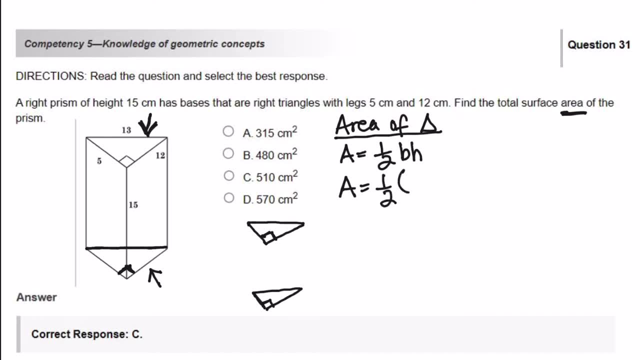 the height, um, so i'm gonna put five times twelve, okay, so that's what we have here. we have a five, we have a twelve and it's for both of them. now, when i do this formula here, this is only one of the triangles. so to do this math, i'm gonna go. 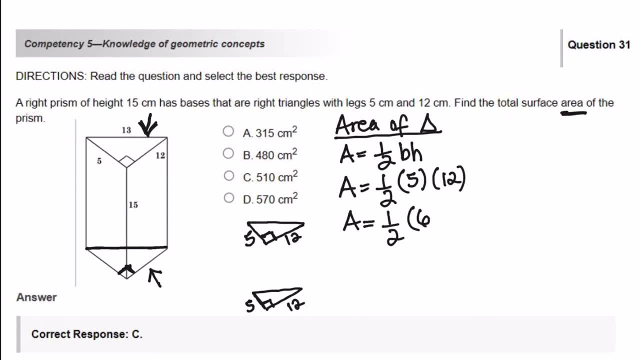 ahead and say one half and five times twelve is sixty. now, this is really half of sixty, so the area of the triangle is going to be thirty. however, you have two of them, so i'm gonna multiply this by two, and so the area is going to be sixty, and in this case, square centimeters. 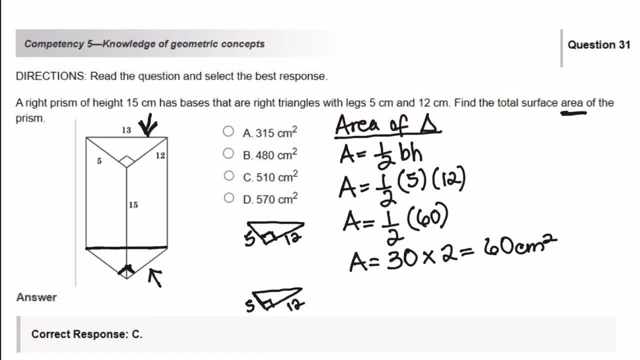 okay, so, um, so far, when we talk about what we've covered so far, we've covered the two triangles. so i'm gonna put, i'm gonna keep a tally over here for our total. so let's put total and this is going to be 60.. okay, let's keep going. so i'm going to erase this because i need more. 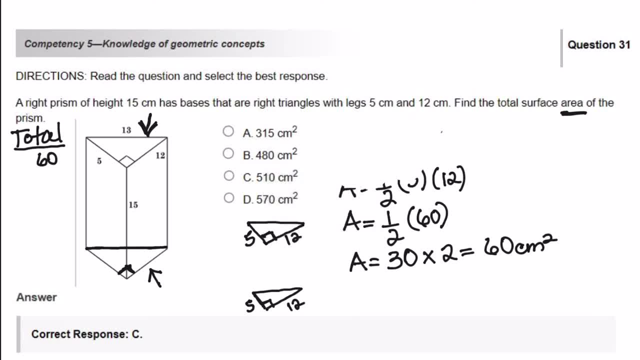 space to write and hopefully you copy that down. so now let's talk about the other pieces of our um prism. so let's pick another color here, okay. so now, if you notice going around the triangle, you have this side. oh, it made a straight line for me. you have this side here. 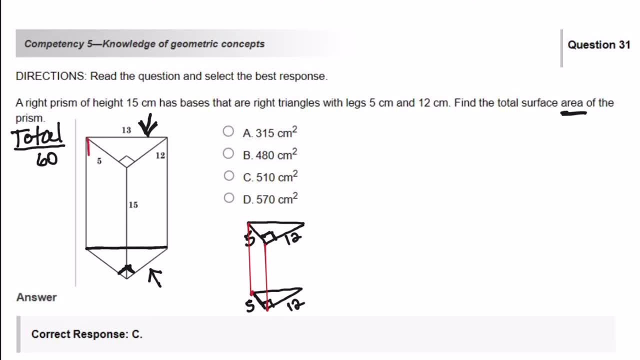 oh, that's beautiful. okay, this is this side here, these two sides right there. all right, so i'm drawing it over here. now that is a rectangle. if i had to draw it as a standalone rectangle, it would be 5 here and 15 for the longer side. so to find that area, area of a rectangle. 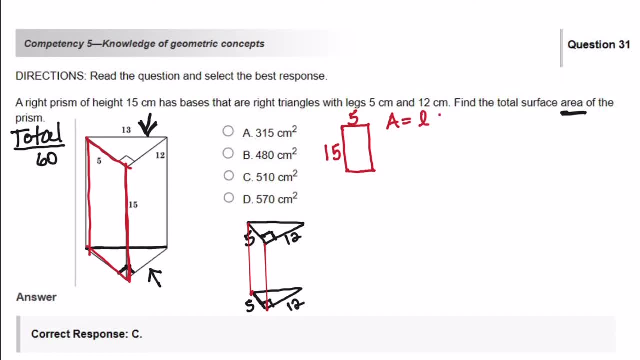 is going to be length times the width, and in this case it'll just be 15 times 5.. 15 times 5, i believe, is 75.. so this triangle would be 75 square centimeters. so i'm going to put this total. 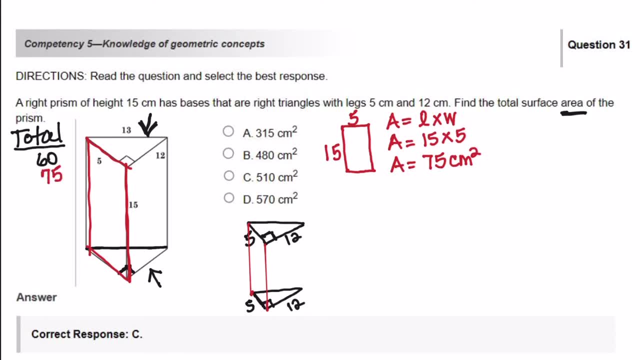 over here. so we now we got 75.. so now let's pick another side of the prism and we're going to draw the other side of the prism. the other side of the prism would go on this side here. if you notice this, is it? so i can draw that from this line and here. 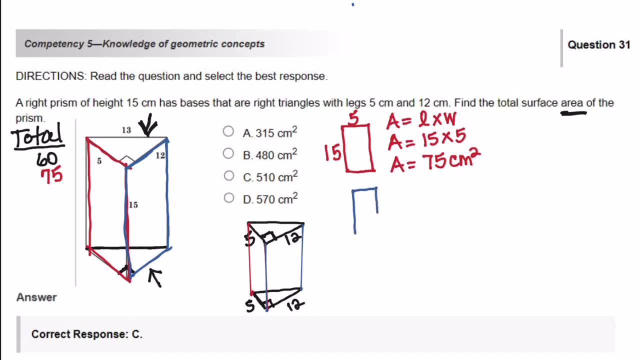 and as a standalone shape, i draw it again. okay, this is going to be 12 up here and 15 here. so this is: area equals length times the width and you have 15 times 12.. now we're actually going to do that math: 15 times 12, you get 10. this is 3, placeholder 5: 1. add it together. 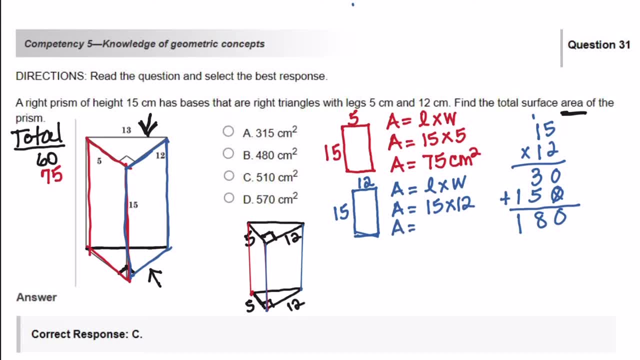 and you get 180.. so this area is 180 square centimeters, so let's add this to our total 180.. okay, so now for the last one. it's only one more piece, and let's put this in a brighter color. so now we have the back of the prism. 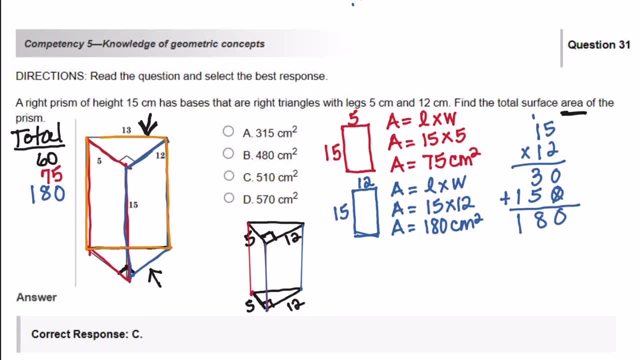 which is this big portion sitting way in the back. okay, hopefully you can see that. hopefully you can see that. if I had to visualize that, or I mean, sorry, if I had to draw that as a standalone rectangle, it would be 13 and 15.. And again, the formula length times the width, This would be 15 times. 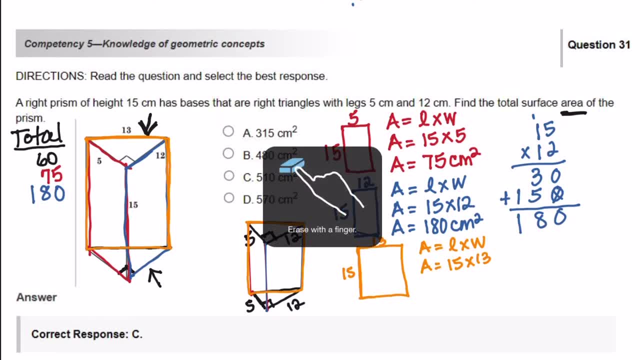 13.. Let's do that math. Let's make some space first. So we have 15 times 13. This is going to be 15, 1, and that's 4.. Placeholder 5, 1.. Together: 5, 9, 1.. So this rectangle is: 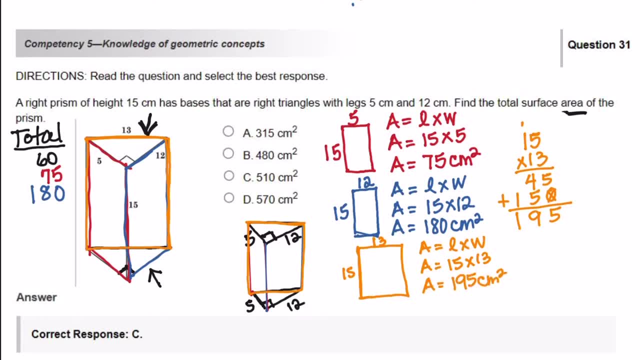 100.. 195 square centimeters, So let's add that on 195.. So now let's add everything together And this would give us our total surface area. So this is 10,, carry the 1.. 7 and 7 is 14,, 14, and 17.. 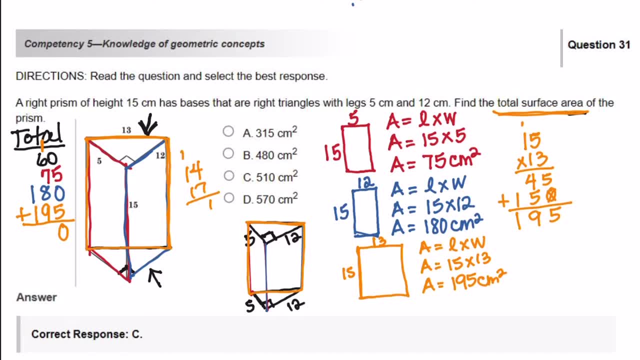 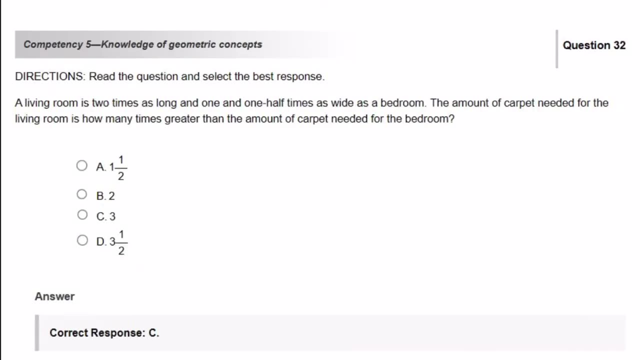 What's 14 plus 17?? Let's see here 11,, 31. And then we have 5.. So our answer is 510 square centimeters. A living room is two times as long and one and one half times as wide as a bedroom. The amount: 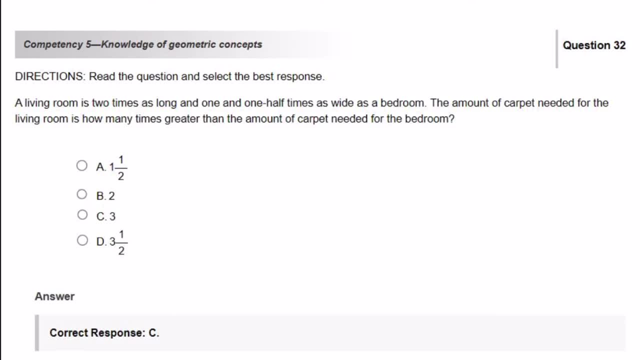 of carpet needed for the living room is how many times greater than the amount of carpet needed for the bedroom. So with this problem here, with any work problem, you're dealing with different types of shapes and stuff. I like to draw pictures, So we are comparing the bedroom and the living room. So we're comparing. 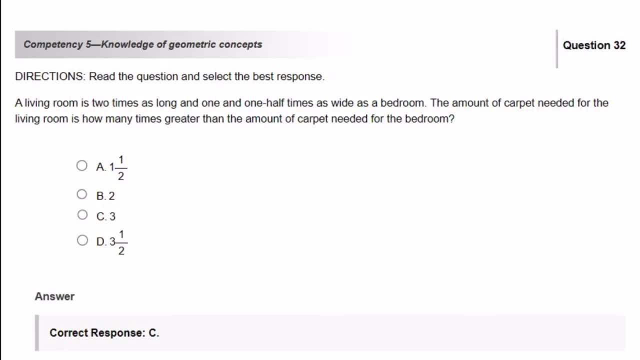 it says how many times greater is the carpet needed. So carpet covers, If you need to that we need to compare the areas. So we're gonna compare the area, because carpet work is a covering of a space, So let's start with the area of the bedroom. 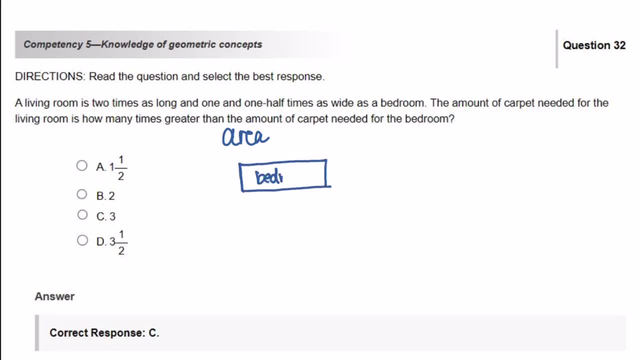 So we're gonna call this our bedroom, And we don't know the width and we don't know the length, So we know, in order to find, areas are going to be: area equals, Wow, exactly length times width, because it is a rectangle. so let's also draw a picture for the living room. 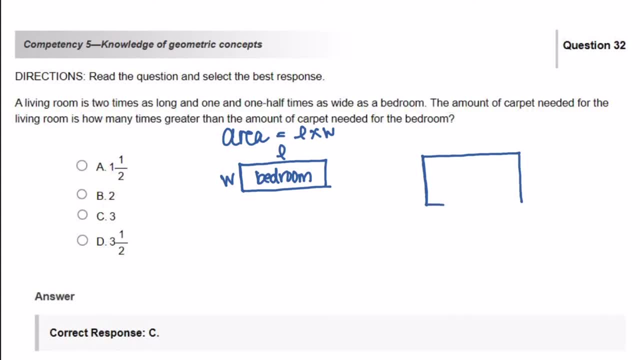 and we know it's a bigger picture, a bigger area, but we don't know how much bigger. so we have the length and the width as well, and this is the living room. however, they say some things about it. it says the living room is two times as long. 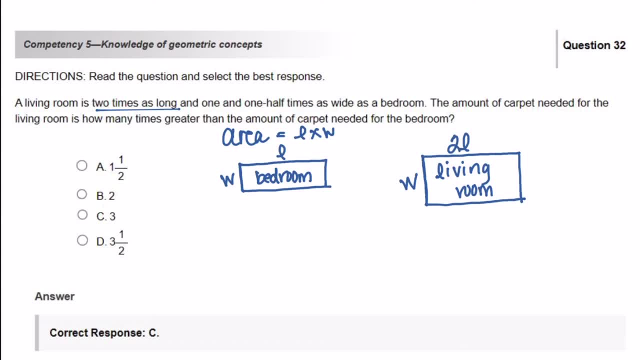 two times as long means i need to put a two here. that says twice the length. and then it also says it is one and one half times as long as a half, one and one half times as wide, excuse me. so we're going to make this one and one half. i'm gonna make it as a decimal: 1.5. okay, so you're comparing. 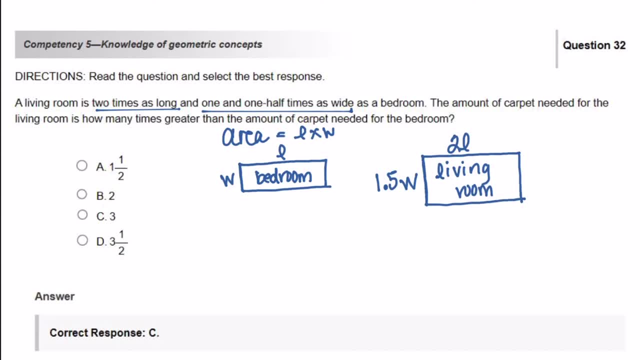 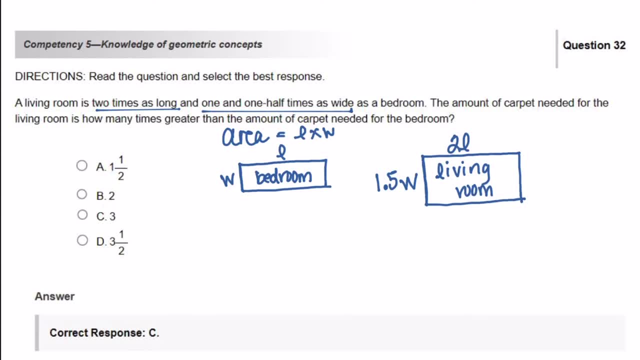 as long as the length as of the bedroom and one and one half times as long as the width of the bedroom. so that's why we put the 2l and the 1.5 w with the dimensions for the living room, and i hope that makes sense. so now, how do you calculate? 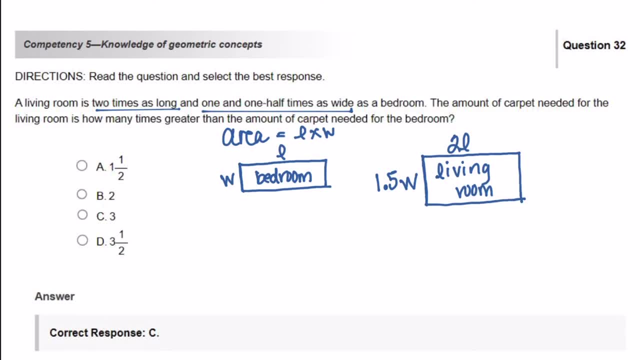 how many times greater it is. so again, you remember the basic formula is: area equals length times the width. well, we just calculated the bedroom, we just wrote it down: l times w. now let's do the same thing for the living room. in this case, it's going to be length times the width, but our l is really. 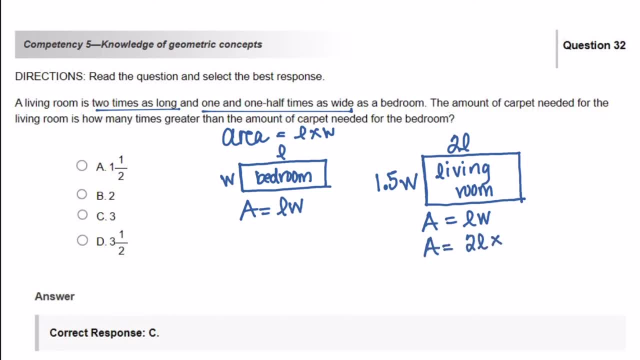 going to be length times the width, so we're going to put 2l times the width, 1.5 w. okay, now let's multiply those two numbers together. 1.5 times 2, it's going to get us 3.0. so this area is going to. 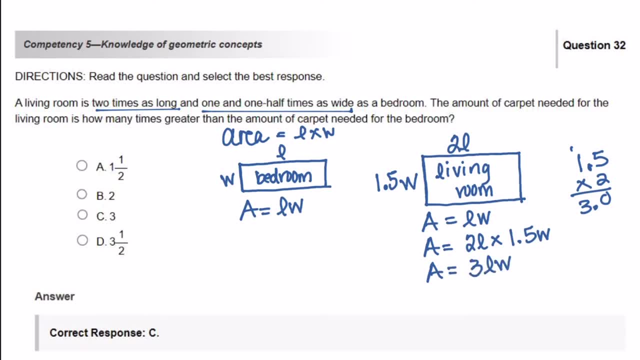 be 3 l w, because we don't know what the length is, we don't know what the width is. so they say how many times greater is the width of the living room? so we're going to put 2l times the width of the living room. 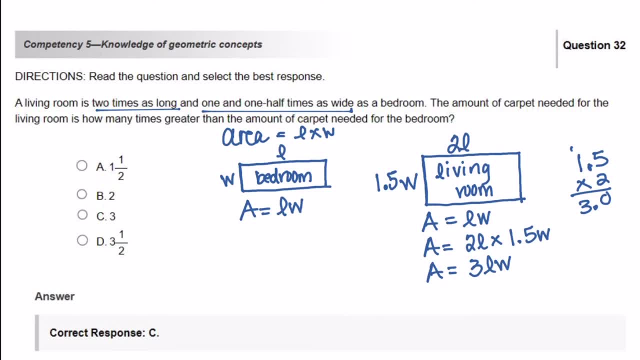 so we're going to put 2l times the width of the living room. so we're going to put 2l times the width of the living room is the living room than the bedroom. and when i say the living room in the bedroom, meaning how many times greater is the amount of carpet needed for the living room? 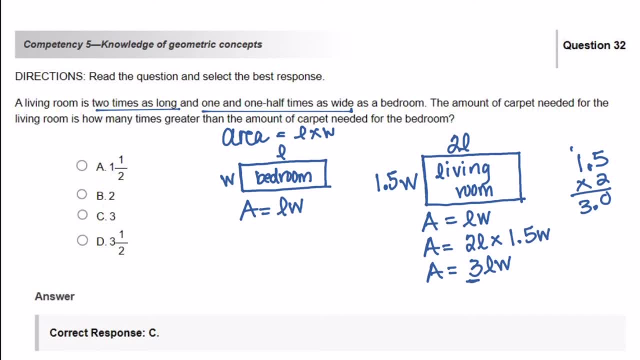 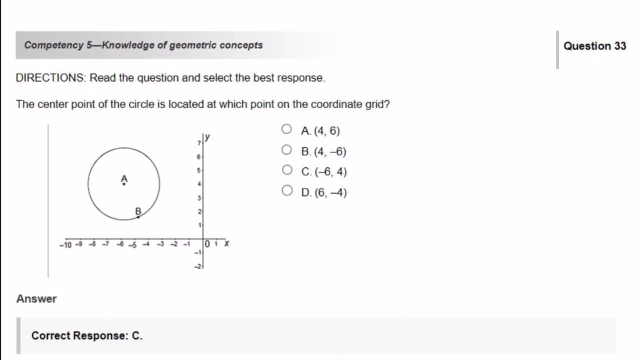 than for the bedroom, and in this case it would be three times greater. c, the center point of the circle is located at which point on the coordinate grid. so in order to be able to read according to grid, you have to know what the numbers mean. so, first off, you have an ordered pair. 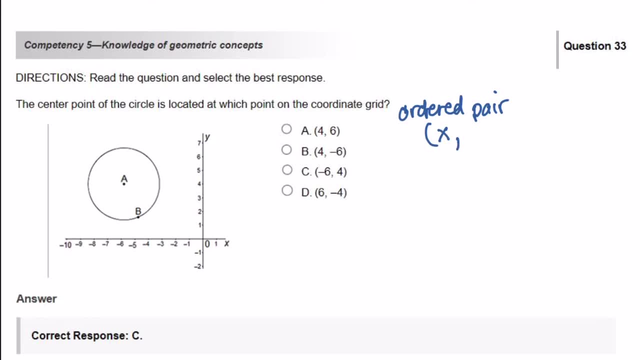 and an ordered pair consists of two numbers: the x-coordinate and the y-coordinate. the x-coordinate is always going to be the first number, the y-coordinate is your second number. the x-coordinate is um, the number you read um going from um left or right, starting at the origin, and the y-coordinate is up or down. so let's look at our picture here. 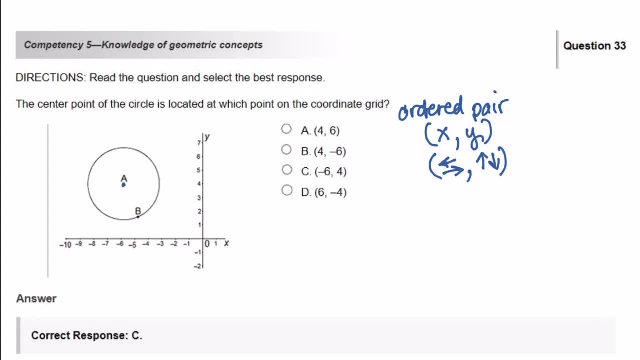 we have a which is the center of the circle and we need to find the pick, the number that um is from the x axis and from the y-axis. so let's draw a line. if you notice that's at negative six, and then we draw a line over here. 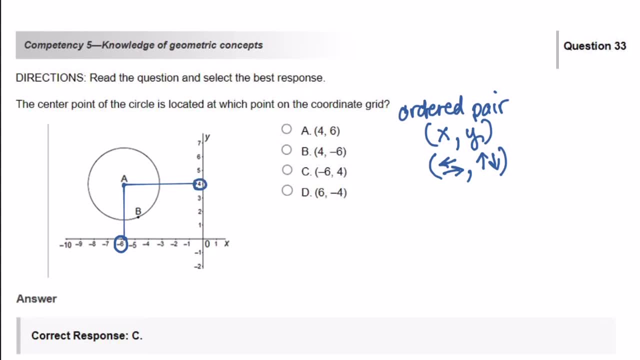 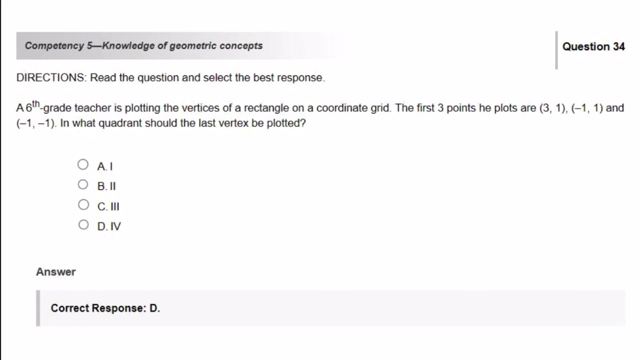 so that's at four. so which one do i pick first? okay, so you always pick the x value first. so this is first and this is the second number. so the ordered pair is negative six and four, which in this case is c. a sixth grade teacher is plotting the vertices of a rectangle on a coordinate grid. the first. 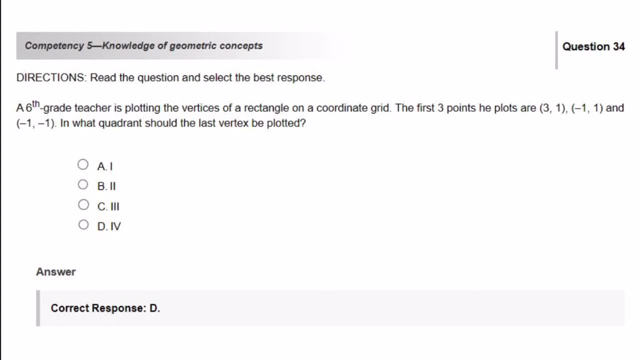 string in the twos be taken over here. number two is going to be negative six upon negative seven. so you use your number to figure out the x value first and first number, and then you pick to pick the next numberl. The first three points he plots are 3, 1, negative 1, 1, and negative 1, negative 1.. 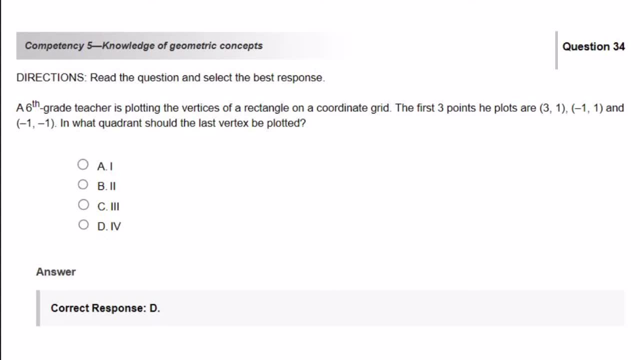 In what quadrant should the last vertex be plotted? So I'm going to draw a coordinate grid and I'm going to plot those points. So we say 3, 1, 1, 2, 3, and a 1. that goes here. 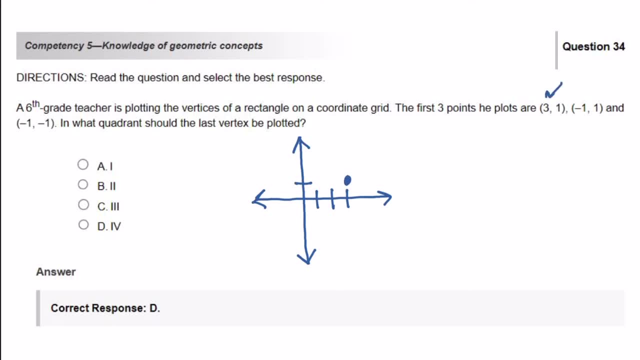 Check. I did that one, And then negative 1 and 1 goes here. I did that one And negative 1, negative 1.. That goes here And you're trying to make a rectangle. so naturally you want to go to this area right here to actually make your rectangle. 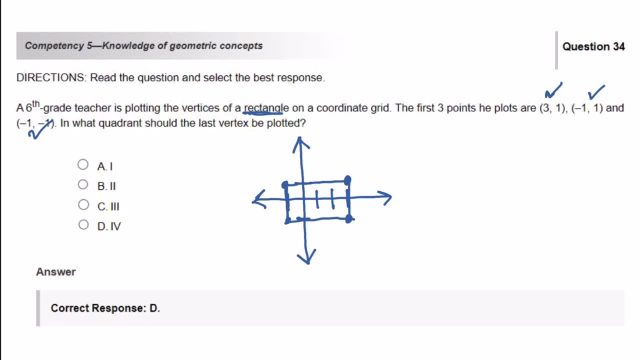 Okay, What quadrant is this in? This is in. You need to know how to list the quadrants. So this is quadrant 1,, quadrant 2,, quadrant 3, and quadrant 4.. And you list quadrants by Roman numerals. so that's why I wrote it like this. 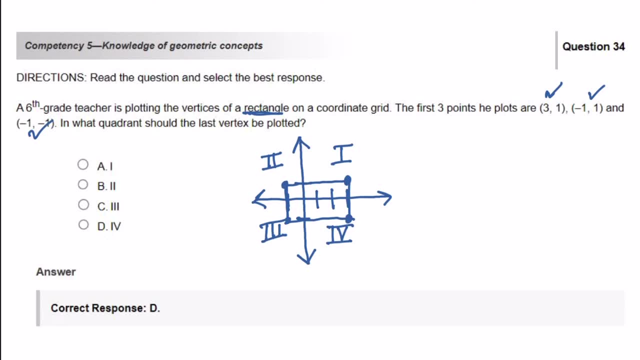 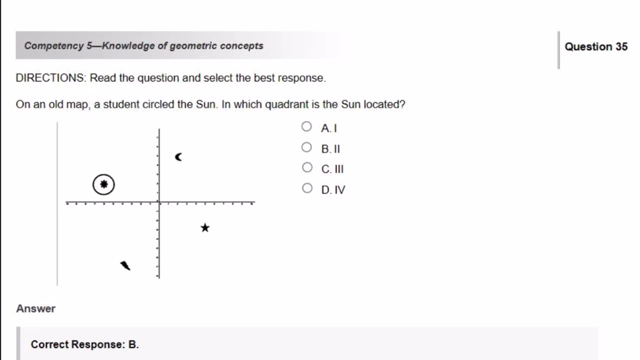 So the quadrant that our last point would go in, or the last vertice would be in quadrant 4D. On an old map, a student circled And which quadrant is the sun located? Again, you have to know the names of the quadrants. 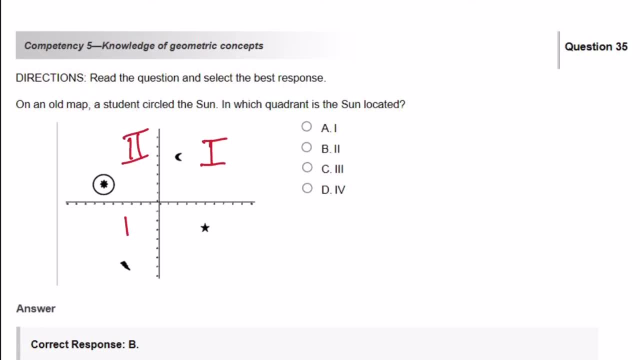 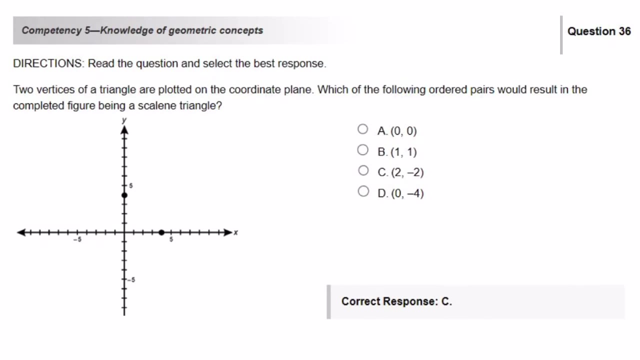 So this is quadrant 1,, quadrant 2, quadrant 3, and quadrant 4.. And the sun is circled here, so that is quadrant 2, answer choice B. Two vertices of a triangle are plotted on the coordinate plane. 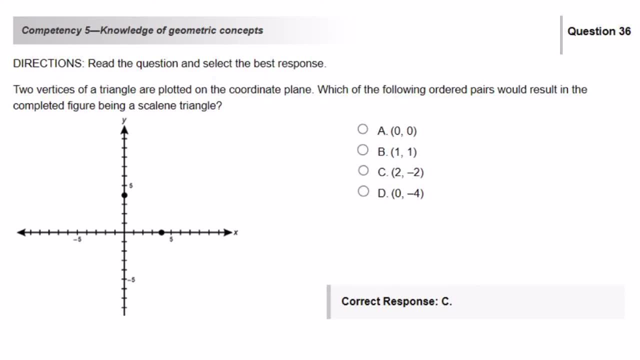 Which are the following order: The first two pairs would result in the completed figure being a scalene triangle. Okay, so in order to do this question, you have to know what scalene means. So when you're working with a scalene triangle, that means that all sides are a different length. 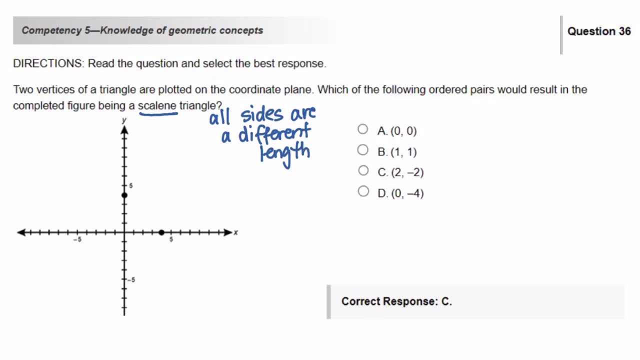 Okay. so let's go through each one of the ordered pairs and let's figure out what type of triangle is created when we plot the different points. So our initial points are the two black dots here. Let me make them bigger. So we have this one here and this one here. 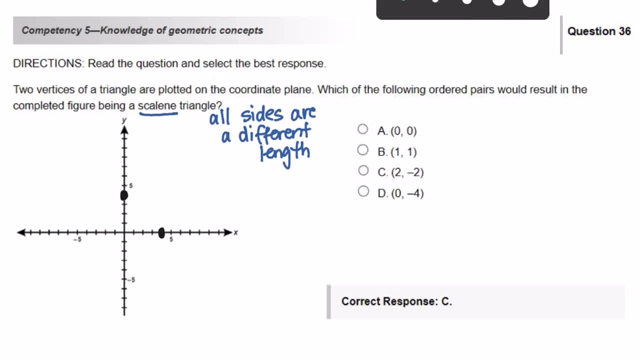 Okay. so if I was to plot the first dot, 0, 0.. I would put it here: Okay, when I draw this triangle, this length is 4, and so is this length. Well, that's already breaking the rule of the definition of a scalene triangle. 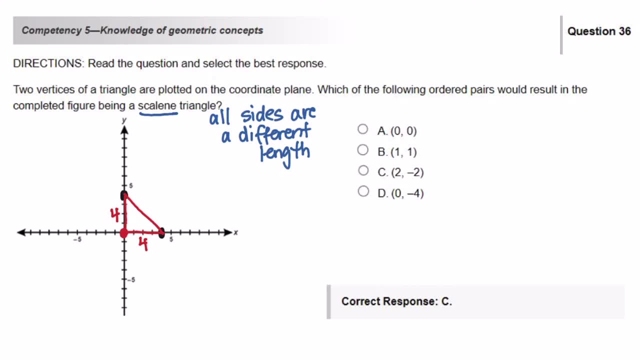 So this would not be the right answer. As a matter of fact, this creates a right triangle, Okay, so let's erase this one And let's put our dots back a little bit bigger and let's do the next one. 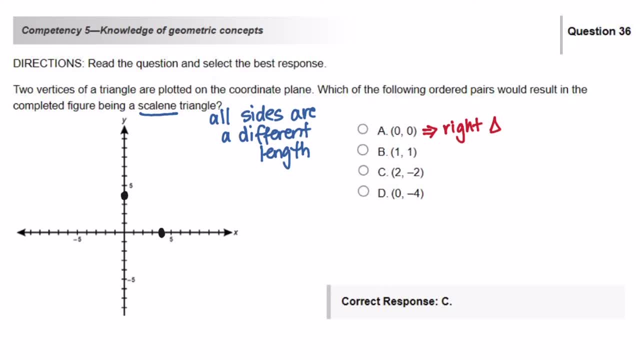 So now let's plot 1, 1.. So we have 1, 1 here, And if we were to draw this triangle, these two lengths here are still going to be the same, So it's like an isosceles triangle. 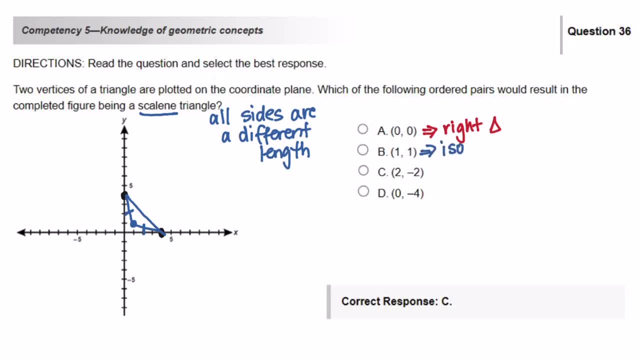 So this would be isosceles, Meaning that two of the sides are the same length. So we're going to get rid of that And, as a matter of fact, the first one is to give it a better name. This would actually be an isosceles right triangle. 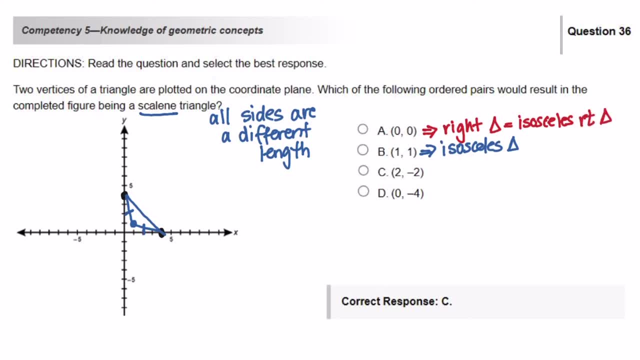 Right triangle. Okay, Let's keep going. Okay, let's get rid of this triangle here. Let's put our dots back here and here And let's go to the next one. So we have 2 and negative 2.. 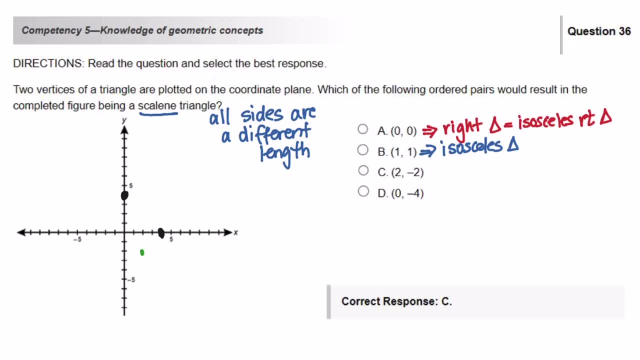 So we have 2 here And then down 2 is going to give me that. So there we go. So with this one here, All the sides are different. They all have a different length. This is short. This would be the first one. 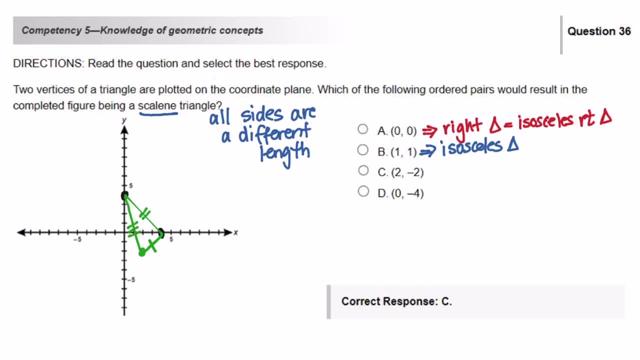 This would be the second one. This would be the third one Because that looks like it's longer. So that meets the definition of a scalene triangle. So, yes, This is the one you want, But let's go ahead and do answer choice D, so that you can see what it should look like. 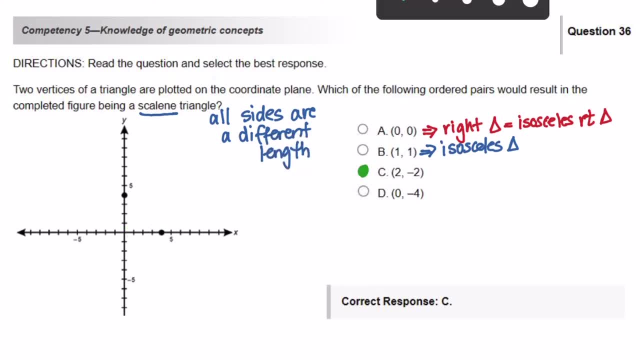 Or what that one looks like. So let's erase again, Let's put our dots back And let's do the last one, Which is 0 and negative 4.. Oh, Wrong one, Sorry, Whoops, Come on Kim. 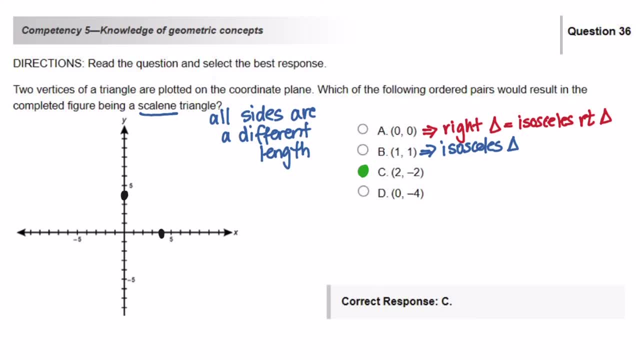 Okay, Let's do that one more time. So let's do the last one, And it's going to be 0, negative 4.. 0 here Go down 4. And so this creates Another isosceles triangle. 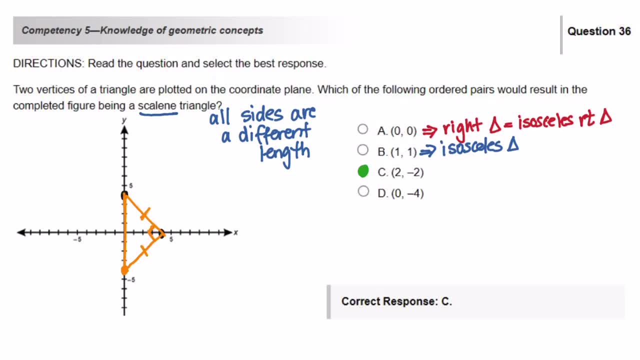 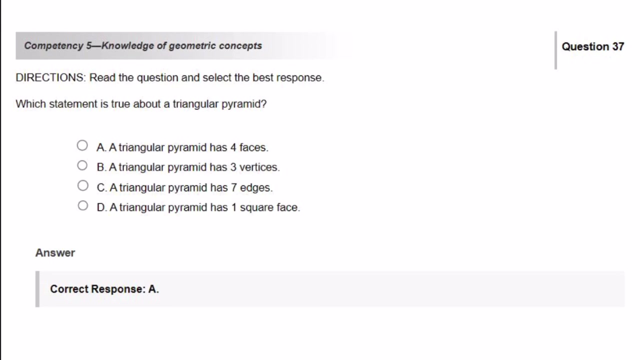 And it actually does create a right angle. So this right here would also be isosceles right triangle. So our answer is C. Which statement is true about a triangular pyramid? First off, let me draw a triangular pyramid for you. 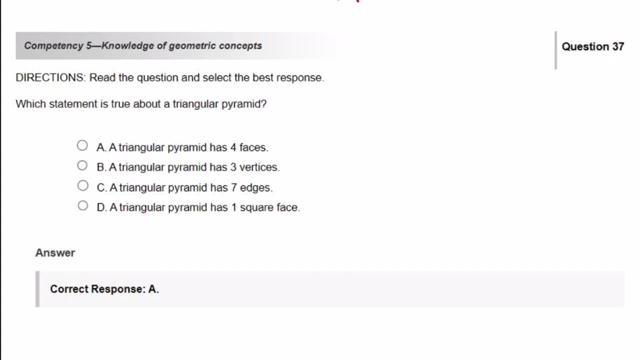 A triangular pyramid means that you have a pyramid and the base of the triangle is Sorry, The base of the pyramid is a triangle. So this is going to be my base of the pyramid And then I'm going to attempt to draw the rest of the pyramid. 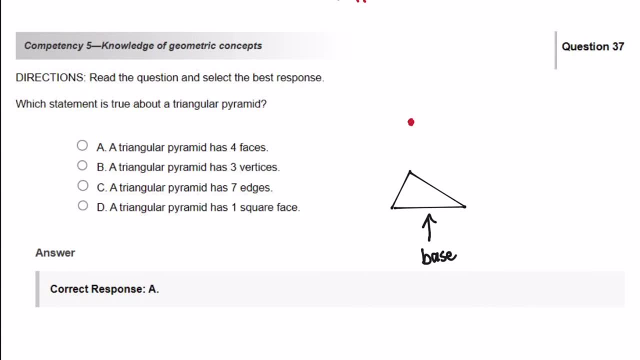 So I'm going to put a dot here And let's draw the rest here, here and here. Okay, So this is my triangular pyramid. The base is the triangle in the black And then up top is the pyramid portion. 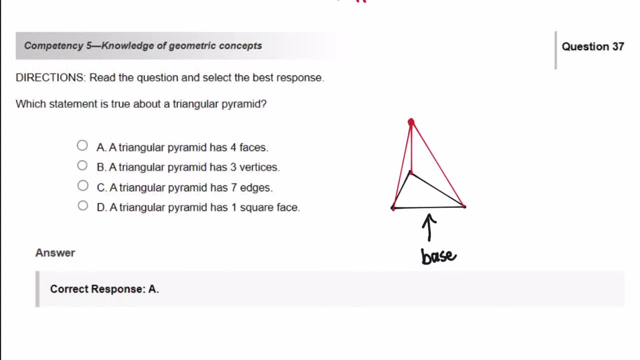 Okay. So anyway, let's go through and make sure we understand what they're asking. So it's. It says a triangular pyramid has four faces, And that is true. So let's count the faces. We have this one here. 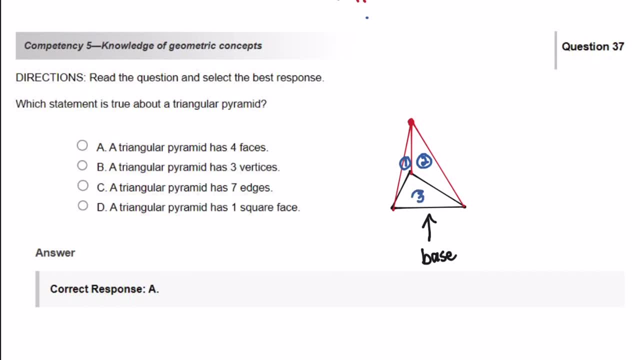 Two: The base is a face, And then this one right here in the front. It might seem a little odd, But this front one facing everyone, This big one here Would be face number four. So yes, That is correct. 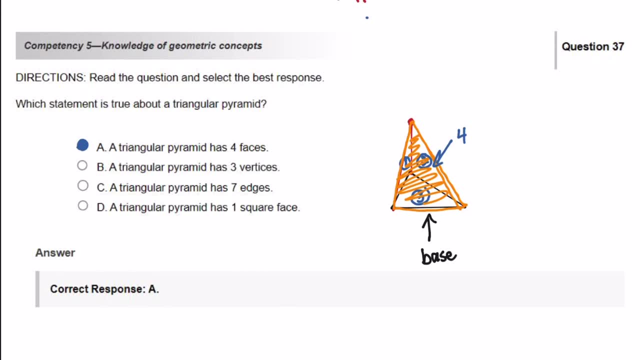 But let's go through and talk about the other pieces that they have here. It says it has four vertices. Vertices are just the vertexes, So you have. Let's do this in a different color. We have one, Two. 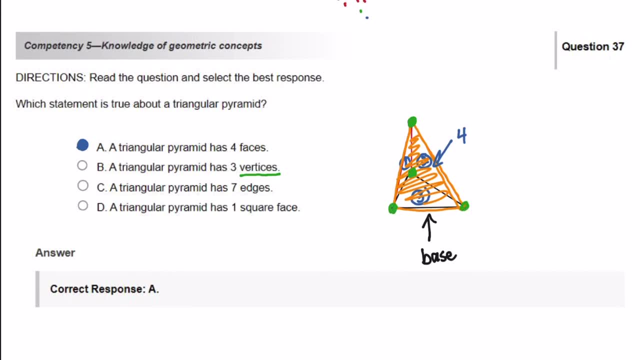 Three, Four. So there are four vertices, Not Three. Okay, Now let's talk about the edges. Let's do that in a whole, nother color. So for the edges, Let's count them. We have one. 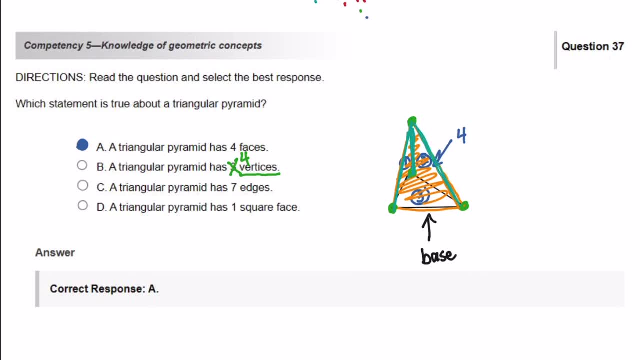 Two, Three, Four, Five, Six. So there are six edges, Not seven. And then it says: a triangular pyramid has a square face. Well, none of the faces on here are squares, So that doesn't work either.